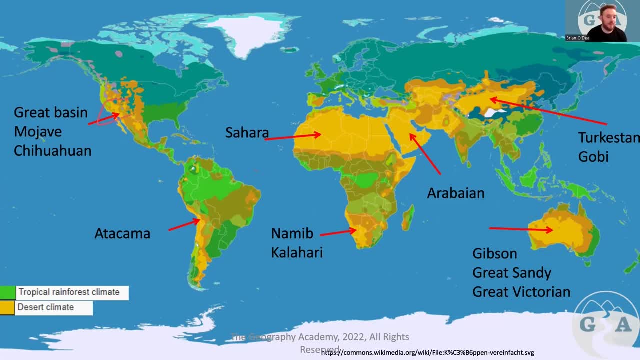 the Gobi desert up here and Mojave desert and other ones, other minor deserts up that area. So we can see similar traits like they're along similar lines of latitude going across the earth, like at the equator we see tropicals. We do see similar characteristics and traits like 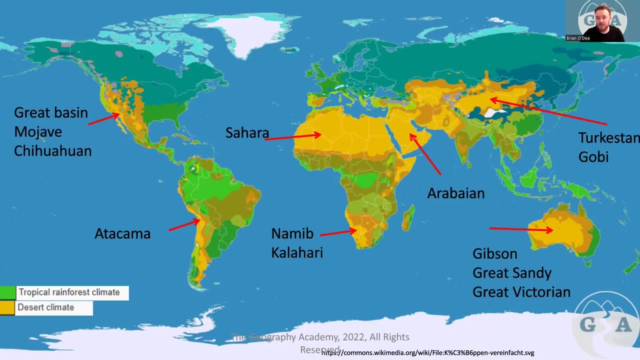 similar lines of latitude, for example. We also see, yeah, similar areas as well, similar distance away from the equator, for example, or near enough, And some of them then are a little bit more north. Some of them, then, are a little bit more south than we would. 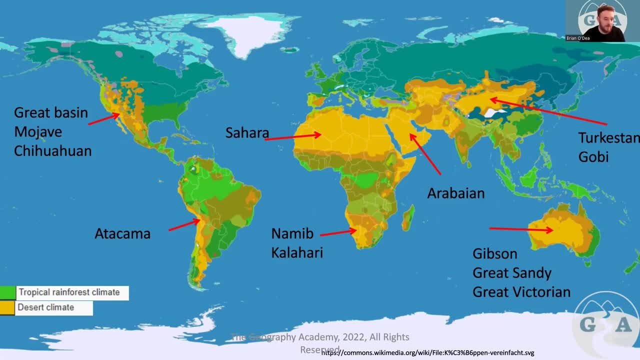 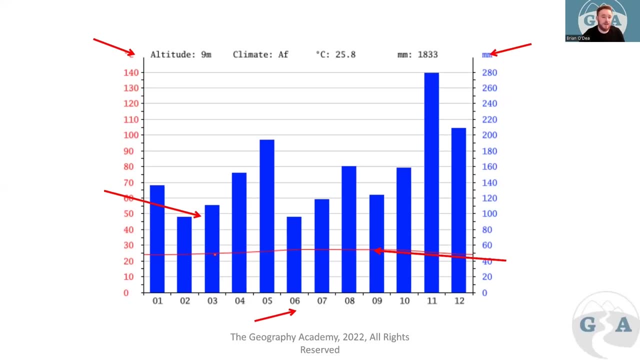 expect perhaps- And yeah, there's certain reasons for the those differences as well. So, in both areas. In both areas you can see the tropical desert. The desert has a very similar landscape to North America, but it's pretty similar. is you want to be able to look at a climate graph? so let's have a look here we have a very basic. 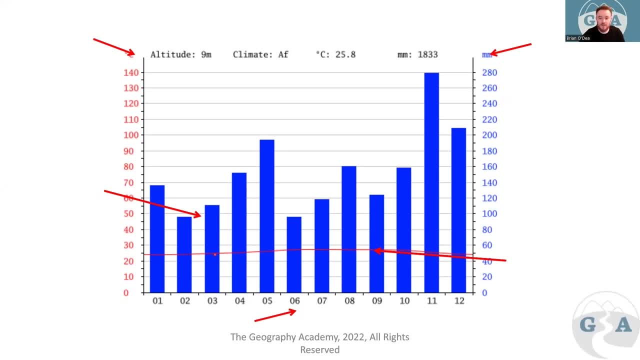 climate graph. we've got degrees celsius on the outside and we've got millimeters in the blue on the other side. we have a right line going through and a line graph and then we've also got a blue bar chart. so you should be able to guess which is which, because the top one on the 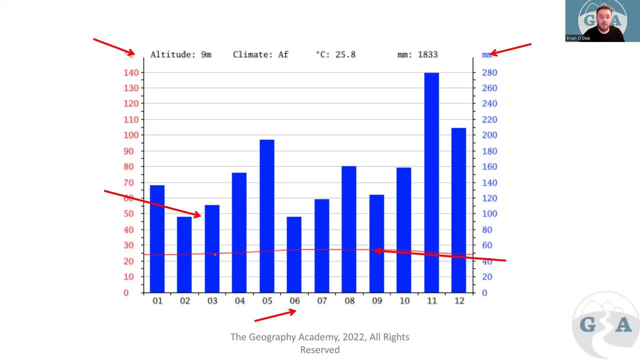 red one is saying degrees celsius. the blue one is saying millimeters. so if you haven't come across them before, let's have a quick look through. so temperature is going in in degrees celsius. precipitation is represented then as the bar chart. we see millimeters as the measurement for. 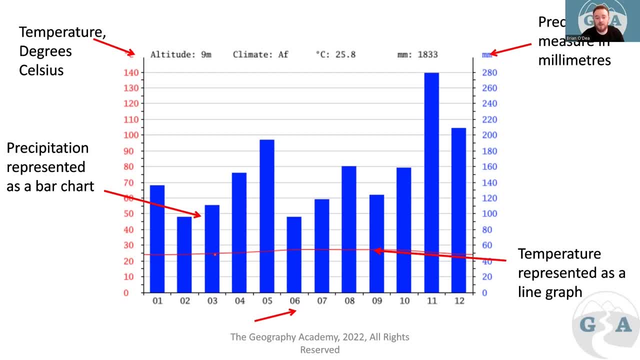 precipitation and the temperature then is represented by the line graph. months of the year are along the bottom start from january, on the first month, to december on the 12th. so this is going to be a tropical rainforest. the characteristics are there to be seen. 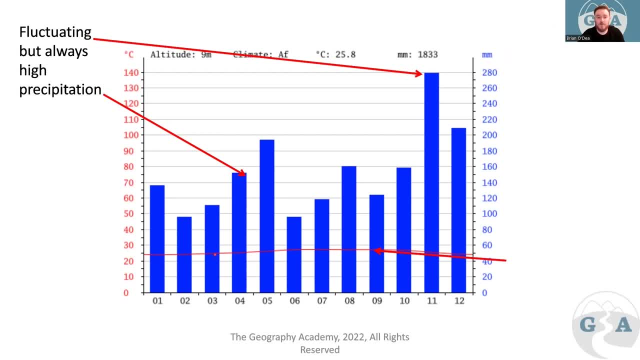 so we have a fluctuating- but you almost always high precipitation. now, if you don't have anything to compare this to, we will in a moment to see just how high that is. so we can see that the maximum in this region could be up to as much as 280 millimeters per month on average. we also see that the temperature stays very consistent. 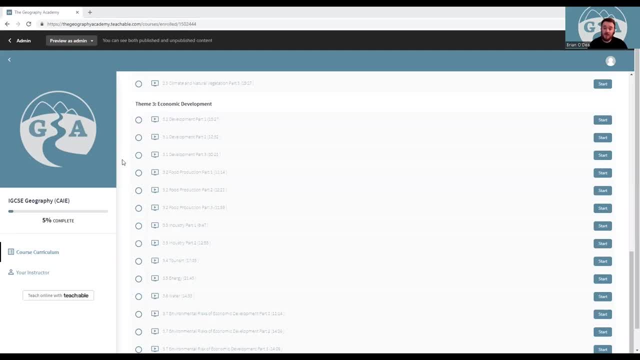 between like 20 and 30 degrees, as always. if that was useful, like subscribe, and i'll be able to post more videos then, but also if you want the rest of the content, follow the links below and you should find what you're looking for. all right, good luck, guys.